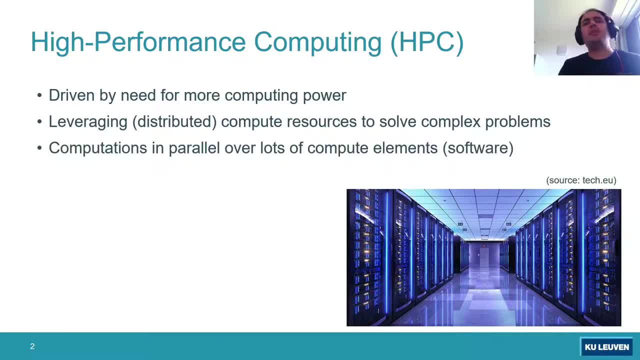 And you know, HBC comprises of software components and hardware components. The software components are usually dealing with performing computations in parallel on lots of, you know, smaller tasks, smaller jobs on different computing elements And, as I said, they are usually distributed. 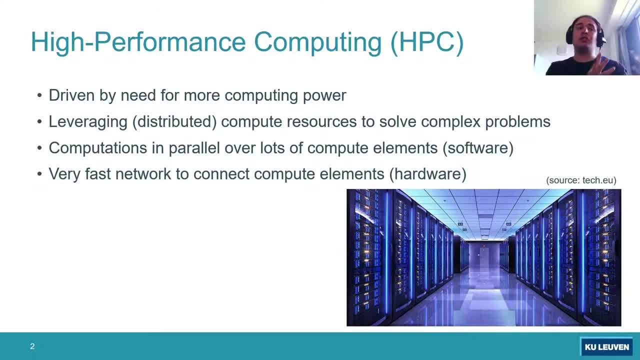 But on the hardware side, we cite, you know, these advanced architectures, structures of CPUs and this kind of stuff. what actually matters a lot is the very fast network that provides this communication infrastructure for these compute elements to interact with each other. And why do we need HPC? That's a trivial question, but, yeah, it has several answers. But 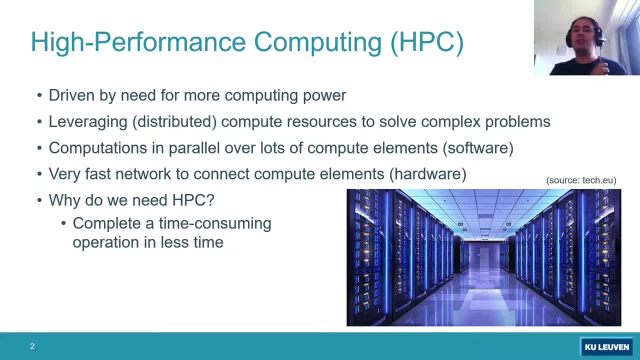 actually, we want a complete, time-consuming operation in less time, or we want to perform a high number of operations per second, And that's actually, you know, a combination of these two is what we are seeking for in HPC, and especially for the things that I want to show you today in. 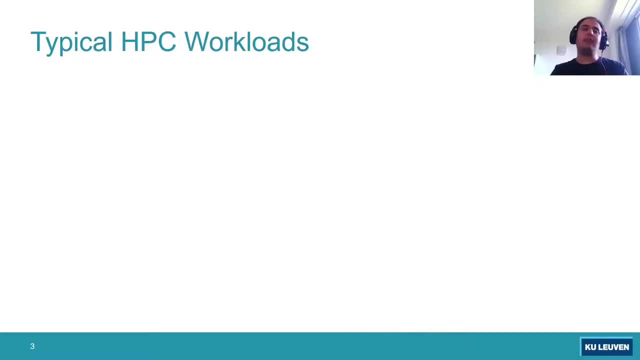 biomedical engineering applications And typical HPC workloads. you know there are a wide range of different applications you can imagine for HPC, for high-performance computing, But you know the The most famous ones are in physics, in astrophysics, also for biosciences, bioinformatics, genomics. 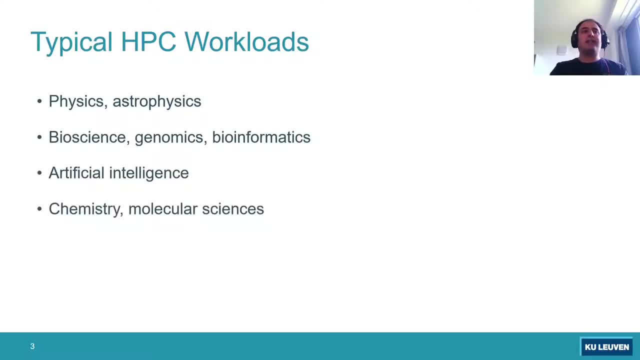 and artificial intelligence, as well as chemistry, molecular sciences- lots of applications in this regard- And then computer-aided engineering, which is actually the topic of this presentation, in mechanical engineering, in aerospace, in biomedical engineering And also computer. 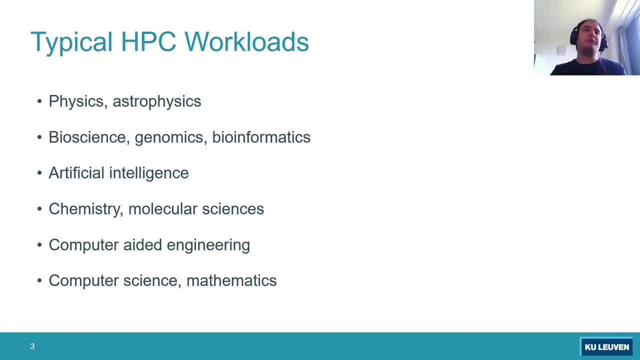 science, mathematics, to develop high-performance algorithms and also solving complex mathematical problems. And then you know, the most famous ones are in physics, in astrophysics also for mathematical problems And big data analytics and financial and economical modeling for risk. 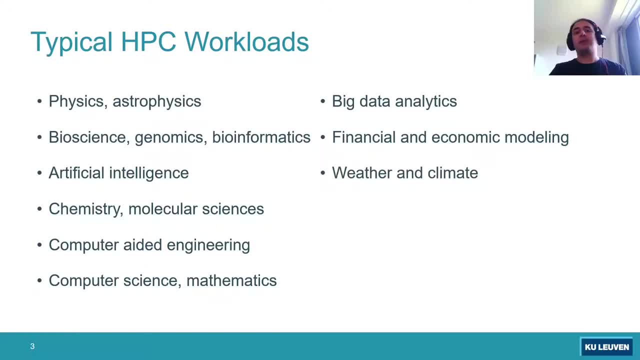 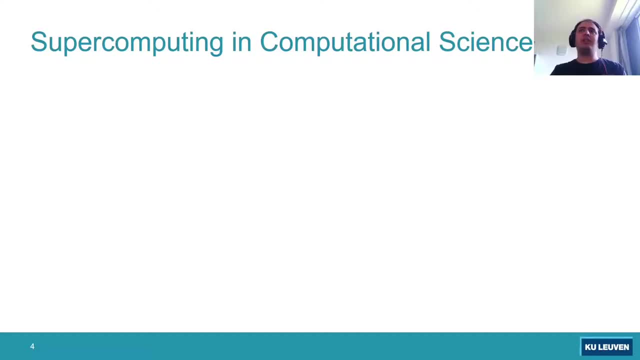 the typical workloads And supercomputing, computational sciences. as I said, it's driven by the need for solving more complex problems in less time And you know, for doing that you can imagine that, yeah, one common solution, one, you know, things that comes from common sense actually. 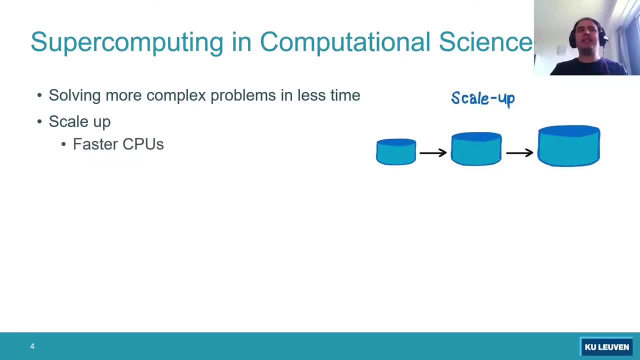 is scaling up, And scaling up means that we employ faster CPUs, larger memories or a more advanced hardware and software tools, And in this way you can easily, you know, increase the performance of applications without modifying the software. let's say, because you scale up the 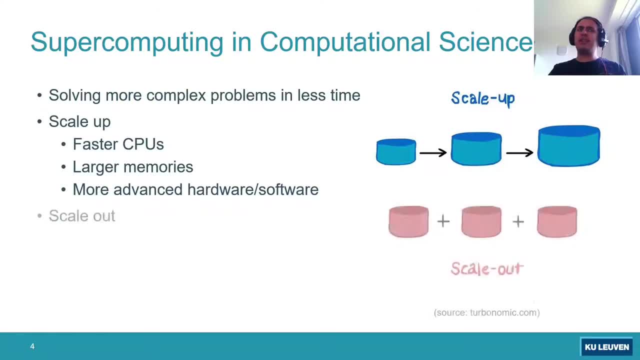 facilities, the equipments. But another technique, which is actually what we are talking about today, is scaling out, And it means that you break your application into smaller jobs, into smaller tasks, and then you can run them in large parallel infrastructure and actually so you can say that, yeah, we have many small to medium jobs, but they are running in parallel. 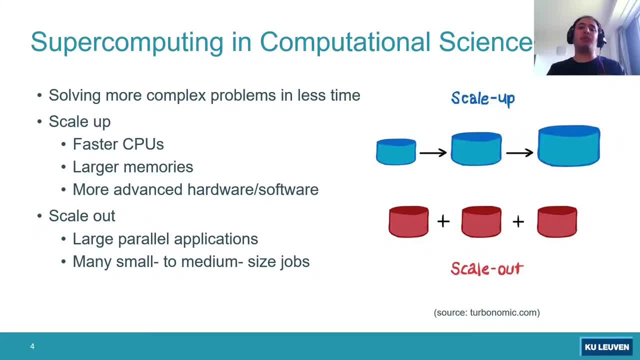 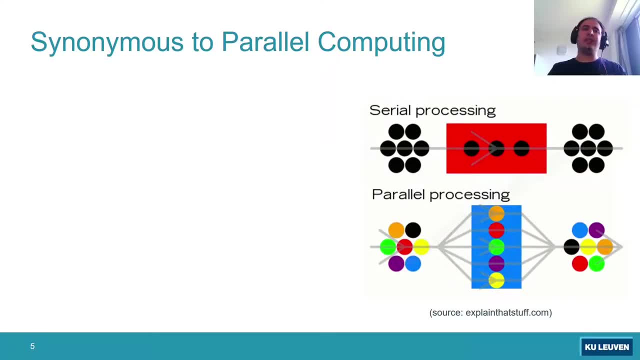 And, as a result, you can increase the, you know, increase the performance and decrease the run time. And yeah, it resembles probably in your mind the concept of parallel computing. So high-performance computing is synonymous to parallel computing And you know, parallelism is available nowadays. 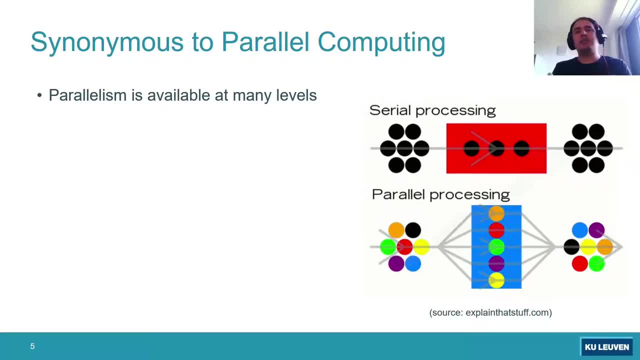 At many levels, even on your laptop. if you have a- yeah, you definitely have a multi-core CPU And it means that parallelism is available to you, even on your local machine or laptop, because you can employ the multi-cores of the available multi-cores to speed of computation if you can. 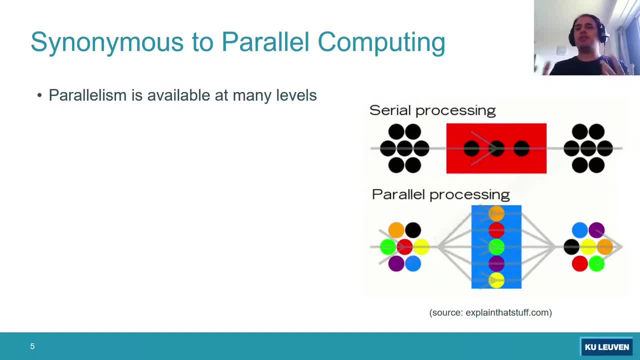 parallelize your computing, your simulations, your models, your codes. But what is really important to consider, to keep in mind, is that all HPC machines are parallel architectures. So if you want to go for high-performance computing, you should go for parallel computing And fundamental parallel architectures. you know. 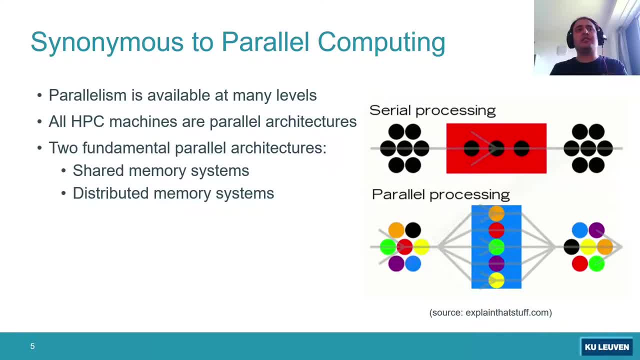 I don't want to go for jargons, but the fundamental architectures are shared memory systems and distributed memory systems. Shared memory systems are like the CPU, as I said, on your local machine, on your local, on your laptop. The different cores have access to the. 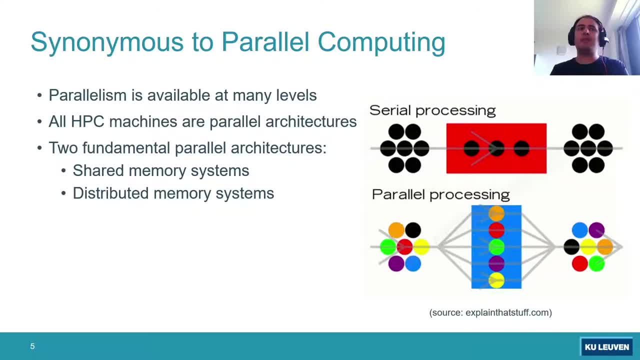 same data because they are on your laptop. So if you want to go for high-performance computing, you are on your RAM, on your memory. But in distributed memory systems you have different CPUs And, as a result, they have their own memory. So it's common to say that the memory is also. 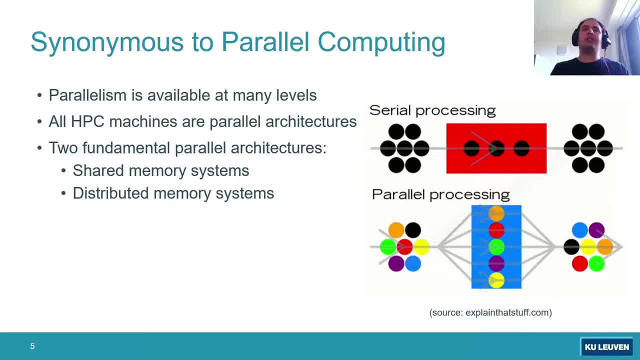 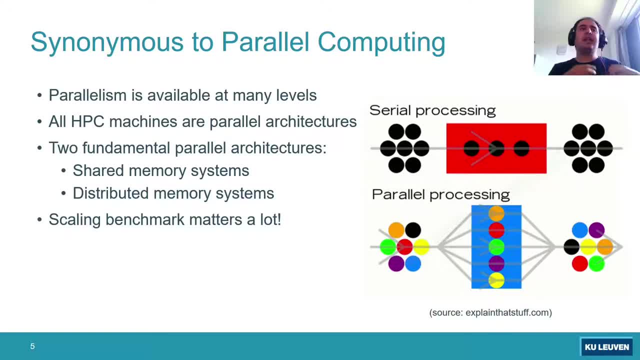 And what matters a lot in HPC is benchmarking and scaling tests to see that your employed techniques for parallelization actually work, And then this kind of benchmarking would help you to improve the efficiency, speed of, and performance of the developed codes. 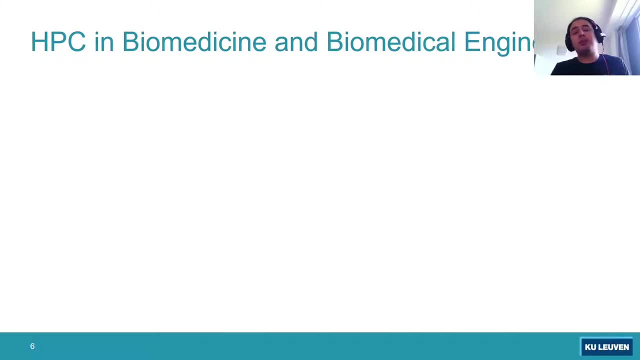 And for HPC and biomedical engineering. you know there are a couple of obstacles And one of the main things is that there are a couple of obstacles And one of the main things is that. you know, in biomedicine and biomedical engineering much effort is put into the model, credibility and 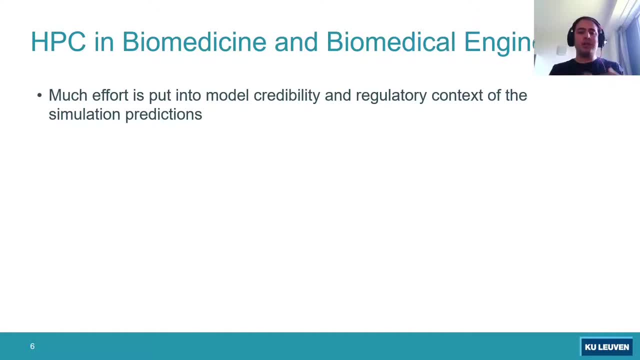 you know, to validating the models and proving that, yeah, these models can work and can be used in clinical trials, for clinical, for medical decisions, this kind of stuff. So this is actually the main concern in simulation, computer simulation and modeling in biomedical engineering And, as a result, less afford, and you know it's put into 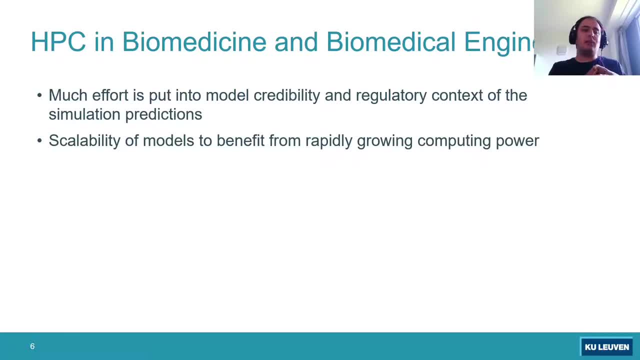 put in the scalability of the models and while it, it has definitely a high gain and for the field and, as you will see in the in the other presentations of this of this session, there are great examples that they have employed the you know HPC techniques to to simulate larger scales and to simulate things that you know. 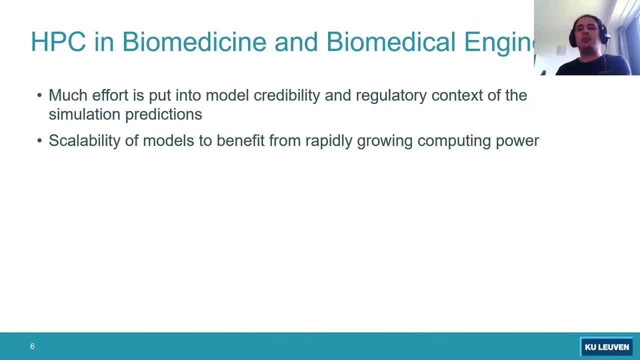 resembles that mimics the physics of the real world much better. but, yeah, generally speaking, scalability of models and high-performance computing things has, yeah, has gained much less attention in in this field, but the potential of impact of HPC can be like employing more quantities of data and parameters, so we 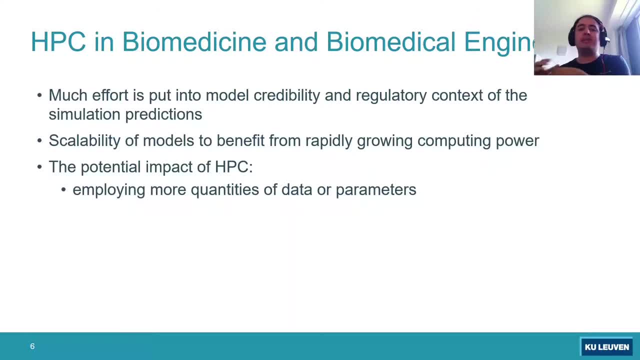 can employ more. we can, you know, take a. you know, take a look at the data and parameters and we can employ more. we can, you know, take a into account more aspects of the real, of the real phenomena that we want. we are going to model, and this will lead to you know, more detailed models and, as a 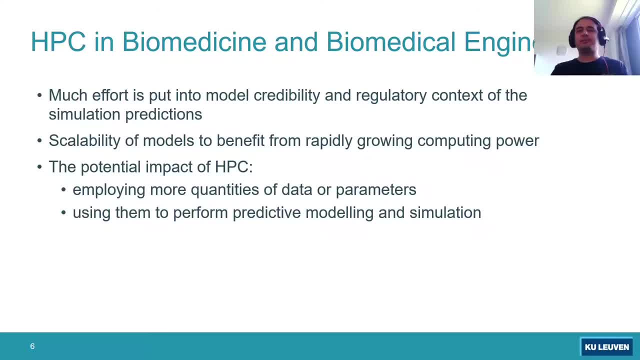 result more detailed simulations, which will be more predicted, let's say, and this will enhance the clinical decision making, because the models would be, as I said, more predictive and they can be employed to make better decisions and deliver better therapies. but what matters a lot in this regard is it will be on shorter. 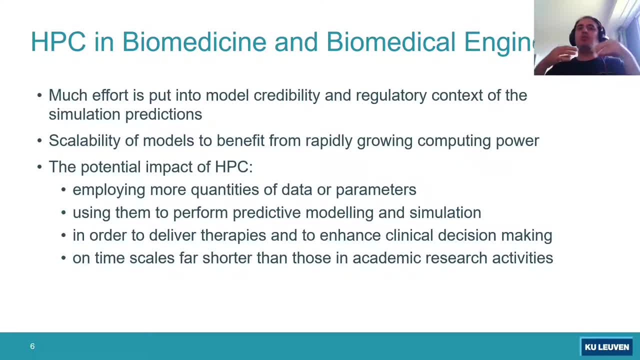 time scales, which means that, yeah, we want to employ more quantities of data and we want to perform, you know, simulation on bigger scales, on you know bigger systems and enhance the therapies, delivery after up therapies and decision-making, but it will be drawn on shorter time scales and decision-making. 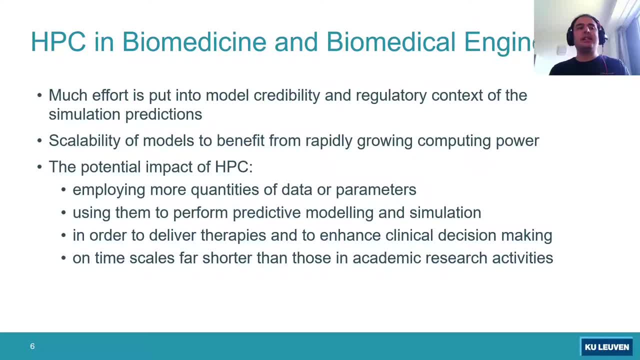 and this is where HPC comes into play, actually, that we want to decrease the progress of antigra are more complicated and we could shrunk the system to the one time and increase the performance. so you will have the results faster, much faster, and in comparison to this cows, that is very. 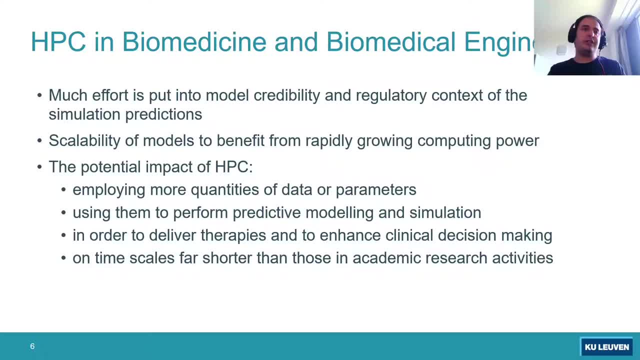 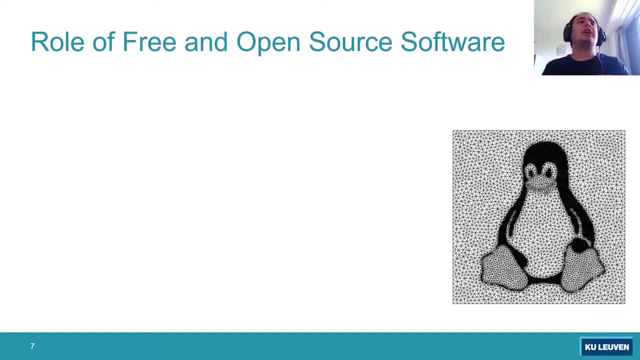 common in academia and also in this way. but as the last note in this general introduction, I want to point out the role of free and a pencil suffer, which is- It's actually undeniable- in the progress of HPC things. So it's very difficult to imagine where HPC would have been without open source tools and open source software. 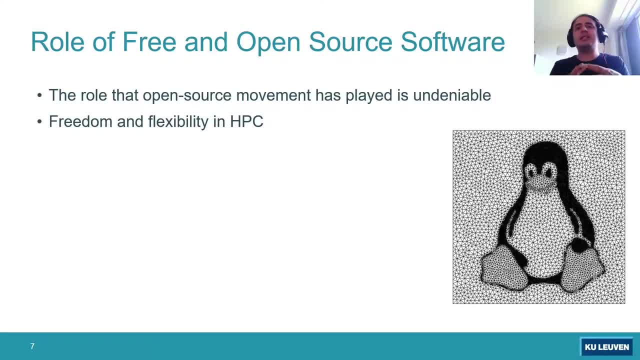 Because, beside the freedom of flexibility in HPC that's quite famous today, This kind of software will bring a flexibility into any field, which is also the same for HPC. But beside this, it's also nice to see that a large number of relevant programs that are being employed in HPC are all open source. 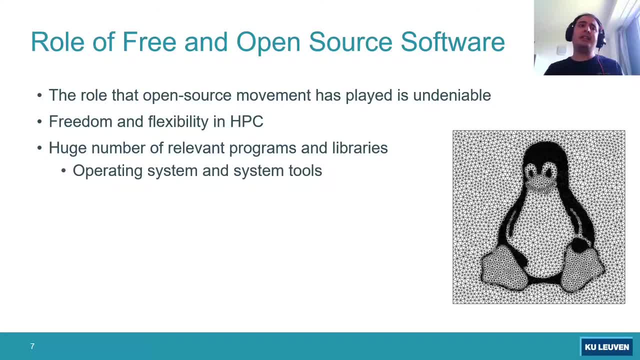 including the operating system, system, tools, low-level libraries, job scheduling and loan balancing system And, more important than them, the high-performance libraries, math kernels, solvers, tools, Petsy Trillinus- all these big libraries that are widely used in numerical computing. 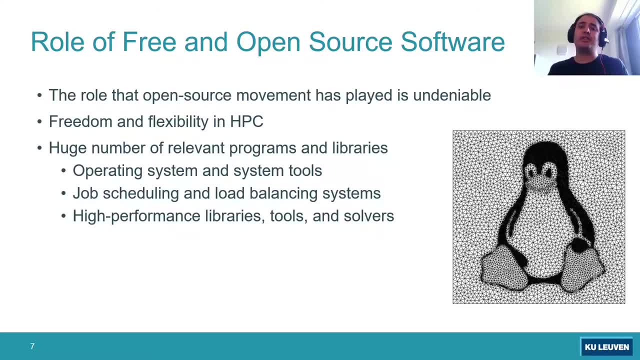 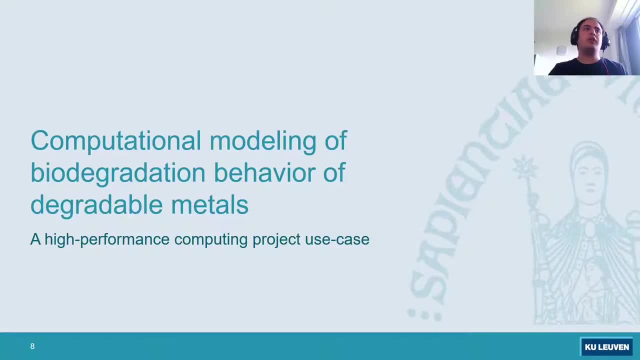 For numerical simulations, for computational modeling. they are all open source, or let's say, 99% open source. So, as an example in this regard, to demonstrate the power of HPC in biomedical engineering and tissue engineering, I want to show you an example of a high-performance computing project that is related to computational modeling of biodegradation behavior of degradable metals. 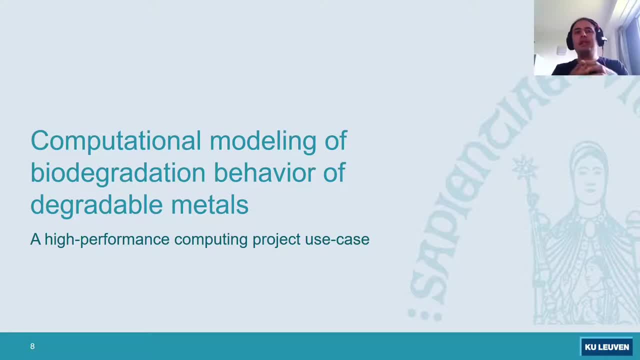 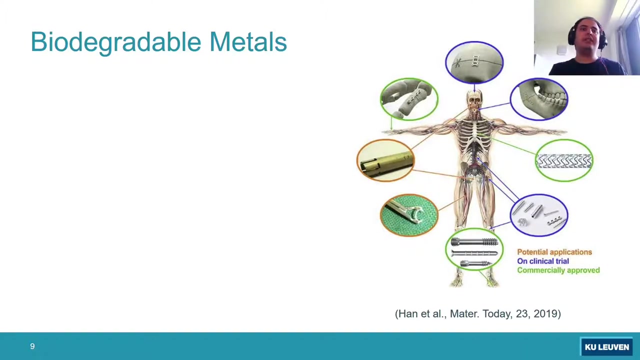 In which to increase accuracy we really need to employ HPC techniques. otherwise we need to wait for ages for simulations to complete. So as a very general introduction to the research to demonstrate its necessity, I can say that when we talk about biodegradable metals, we are usually referring to magnesium, zinc and iron. 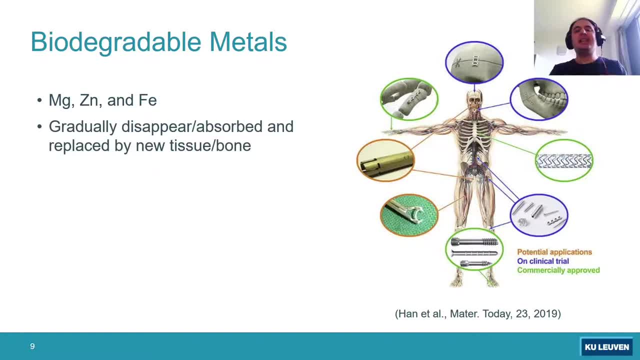 And we mean that, yeah, we put some materials inside the body and they gradually disappear. They get absorbed by the body and replaced by new tissue or bone or whatever that is actually growing there, And they have great mechanical properties, biological properties, but the problem is we need to tune the release profile. 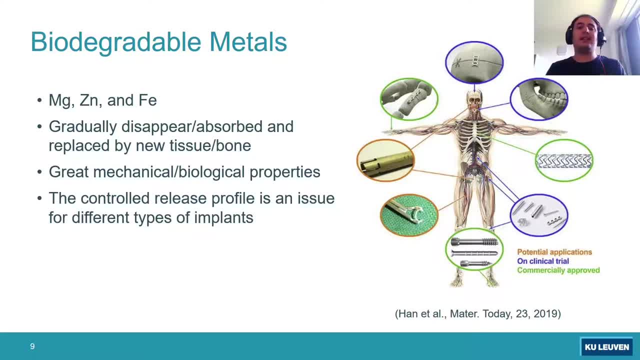 Because, yeah, it's really difficult to predict how they will, you know, they release the material and how they disappear, how they degrade inside the body. So this degradation, So biodegradation behavior, should be optimized and tuned for different applications. as you can see, they have different applications for various fields: for orthopedics, for you know, for dental applications, for cardiovascular things, but the profile should be optimized. 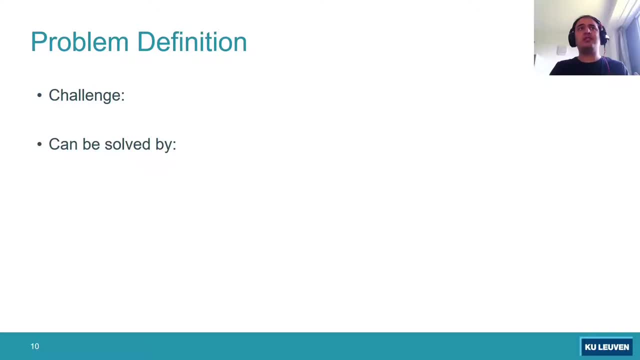 So the challenge of the research, the challenges that the research is trying to address, is tuning biodegradation rate to the generation of the new tissue, And it can be solved by constructing a mathematical model of the biodegradation process that can be coupled with a tissue growth model, so we have the degradation of the material and the growth of the new tissue. 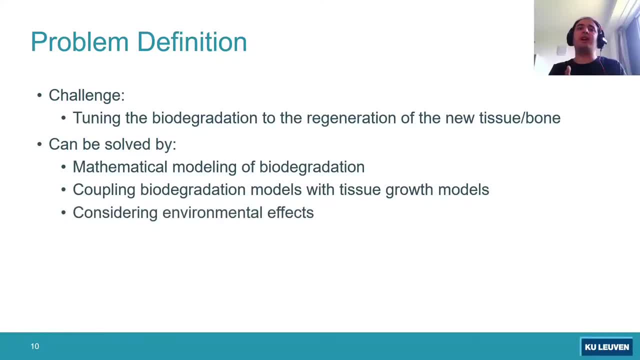 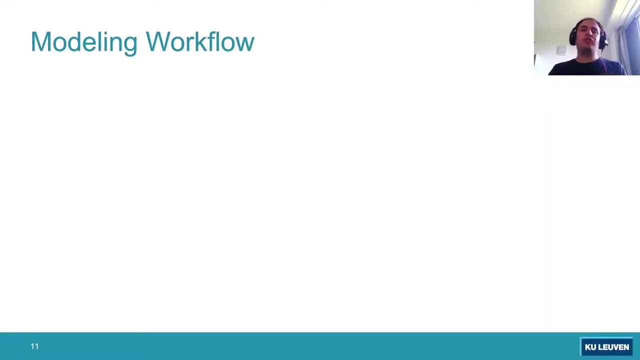 And we should consider the different environments, including, like the in vitro environments in the lab or in vivo environments, in vivo situations inside the body. So the models should capture these situations In order to do that. the workflow- yeah, this is a common workflow in most of the, you know, computational modeling projects, that the underlying sciences are converted to mathematical models and then mathematical models to computational models. 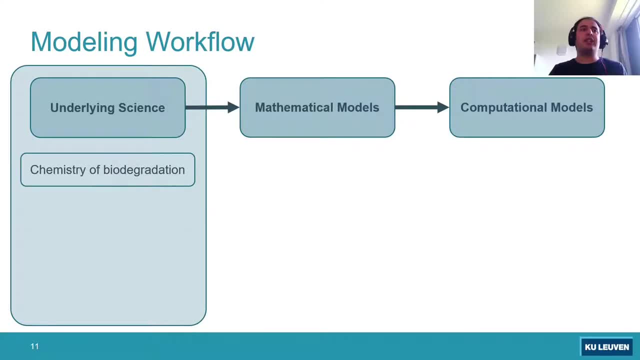 In this project. the underlying science is that chemistry by degradation, The physics of perfusion. because we want to, if you want to validate the models in vitro, In vitro conditions, then we need to consider the perfusion bioreactor setups in which you have a Floyd flow. 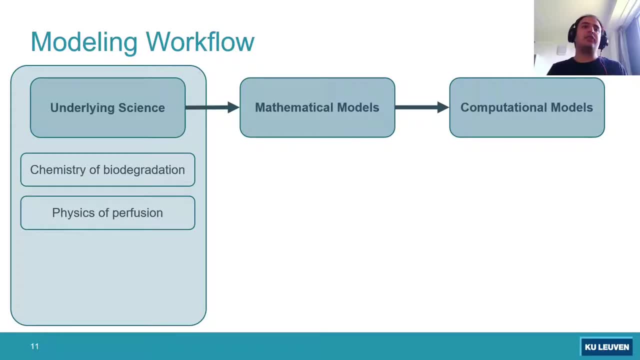 And then this should be considered, This should be considered, And then this should be considered, And then this should be considered, And then this should be considered. it should be taken into account and also the biology of tissue growth. as I say, we want to also capture the biology of the tissue growth and its effects on the 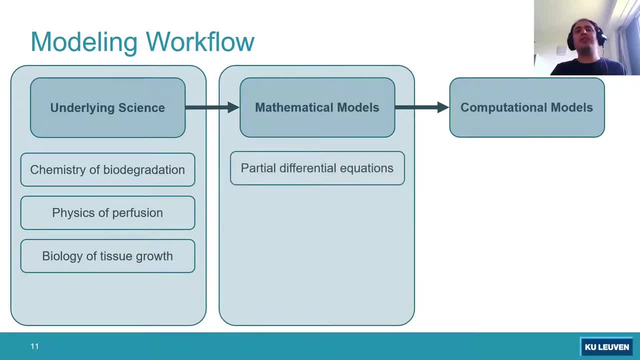 degradation. For mathematical models we have partial differential equations. so this: the underlying sizes are converted to partial differential equations, mainly reaction, diffusion, convection equations- sorry, Navier-Stokes equations- and level set method. and the level set is actually for capturing the way that, yeah, the material degrades. there is a moving interface and then we want to capture it. 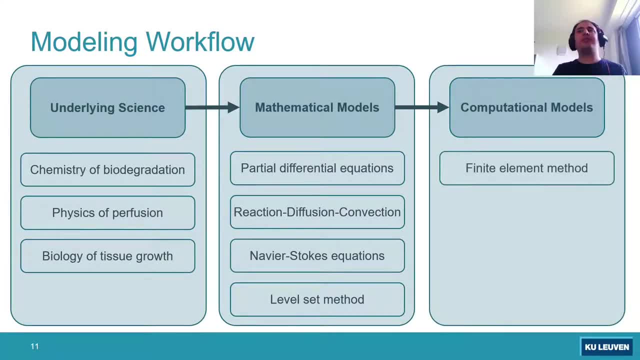 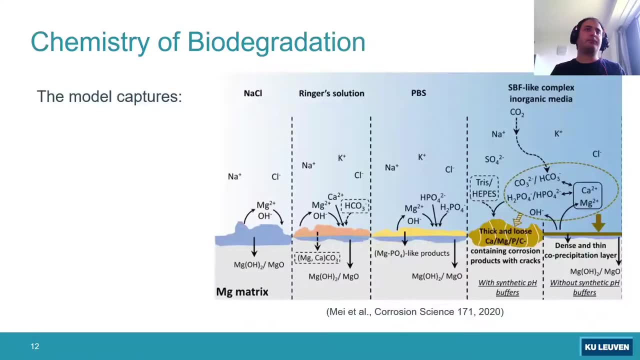 and a computational models is a combination of finite element method and finite difference method, scientific computing libraries and open source solvers. So the model should capture, you know, from the perspective of chemistry, when I discussed this only in this presentation, from the perspective of chemistry, the model should capture the dissolution of the metallic implant. 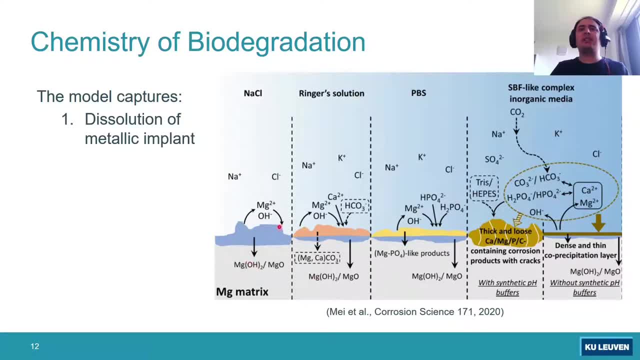 which is actually this part, can see that it did metallic implant in different solutions. You can detect the metallic implant in a different solution from the other part of the body. so and the dissolution of this metallic implant, formation of a protective film which has different composition in different, you know, in different. 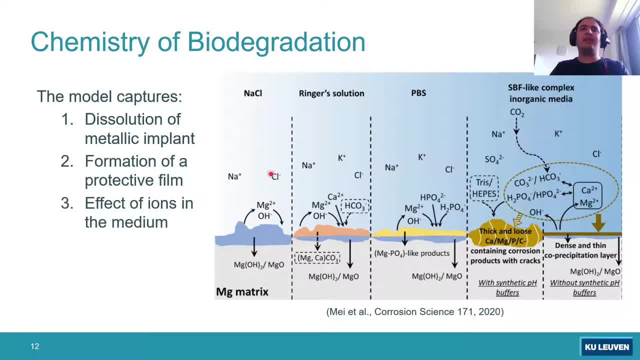 environments, let's say The presence of effect of different ions in the medium. depending on the medium, you will have different ions, different chemical components and they have different effects on this layer and also on the underneath, and also the change of pH, which can be a good criterion to validate the models. 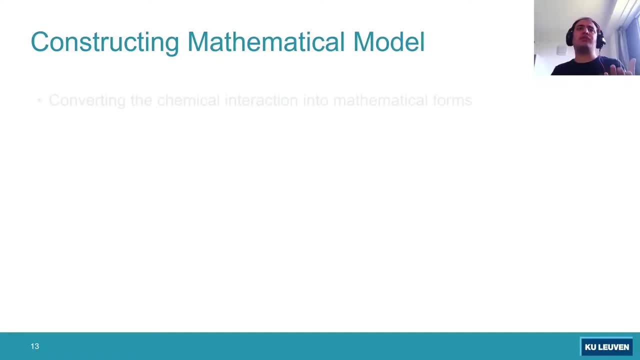 To construct the mathematical models. this chemistry should be converted to the mathematics and in order to do that, we can employ reaction-diffusion-convection, partial differential equations And, as an example, just for magnesium, this is, you know more or less, the form of the. 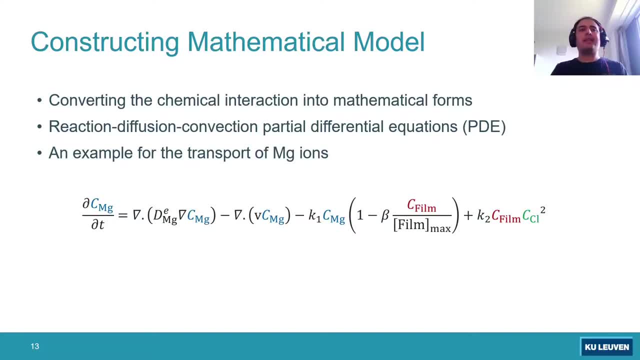 mathematics, the mathematical form of the equations, let's say That's, you know, similar to this. we usually have six, seven, eight, these you know, more or less equations describing the chemistry. So this is actually how magnesium diffuses, how it gets. 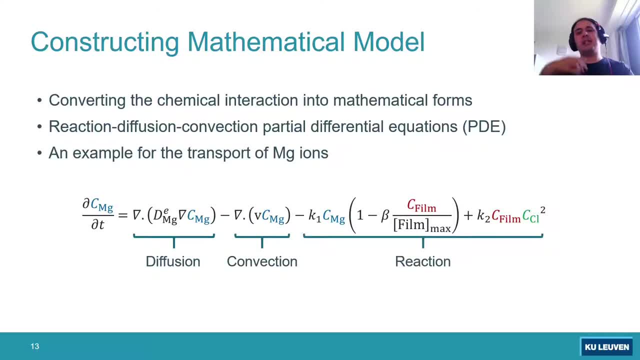 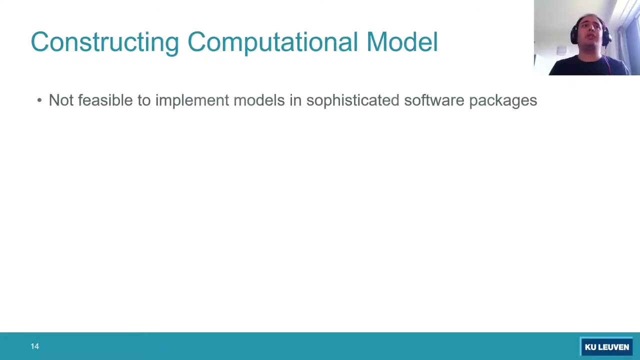 convected, and how it reacts with its surrounding environment and also with different components. So this is the style. this is a form of the mathematical model in this work But, as I said, there are more PDEs In order to construct a computational model, due to the complexity of the mathematical. 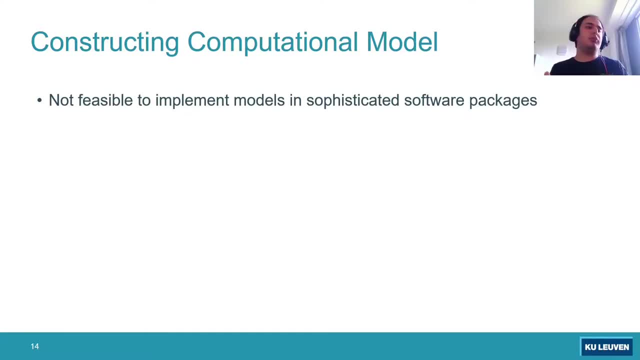 equations and the mathematical model. it's not feasible to implement this in sophisticated software programs and already available commercial solvers like ANSYS and AMBACUS, And as a result, we decided to develop our own solver using finite element method to discretize the PDEs. 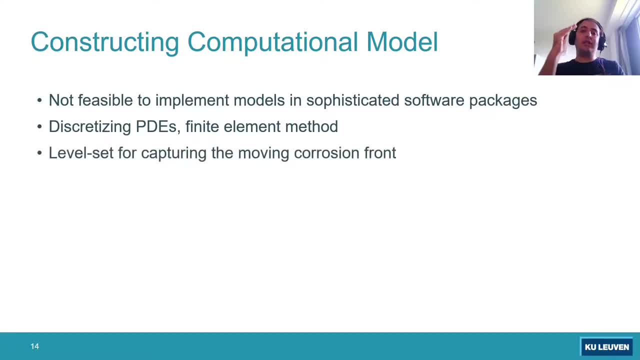 And, as I said, we used level-set method to capture the moving corrosion fronts. So actually by degradation is a sort of corrosion and when something degrades then you see that the interface moves And we use level-set formulation for capturing this. 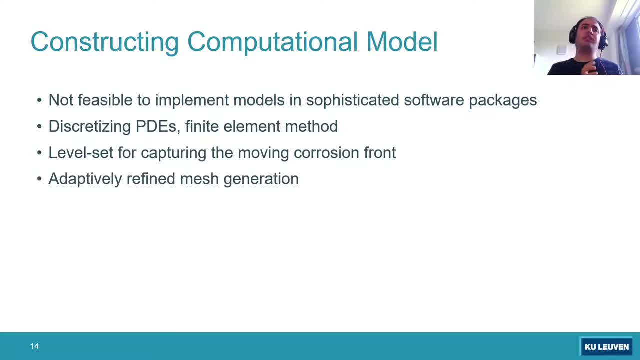 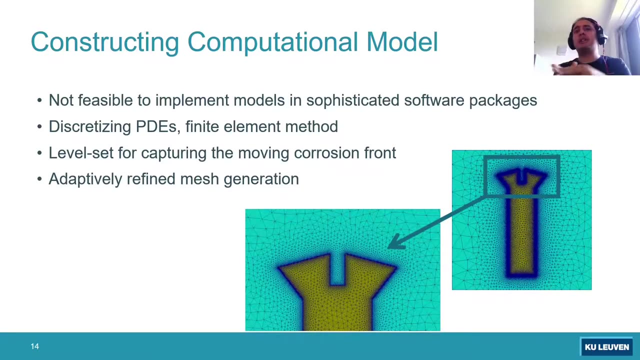 And this is why we need to refine the mesh on the interface, on the moving interface, to increase the accuracy of these numerical schemes. And this is actually how it works that we refine the interface. we refine the mesh on the interface between the metallic parts and the surrounding mediums. In this case, 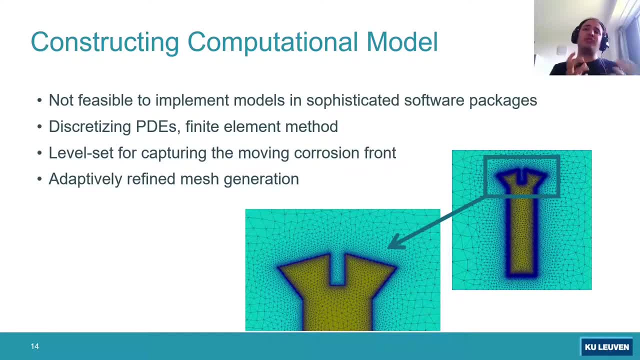 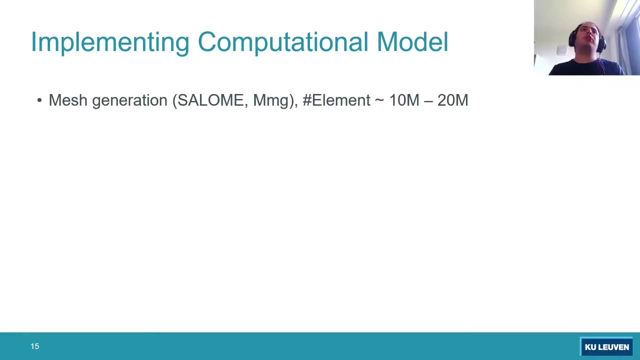 you can see an example in 2D for a simple screw, But in 3D then it becomes very, very intensive because you have millions of elements And that's why we need HPC for this. So to implement a computational model in the mesh generation process. 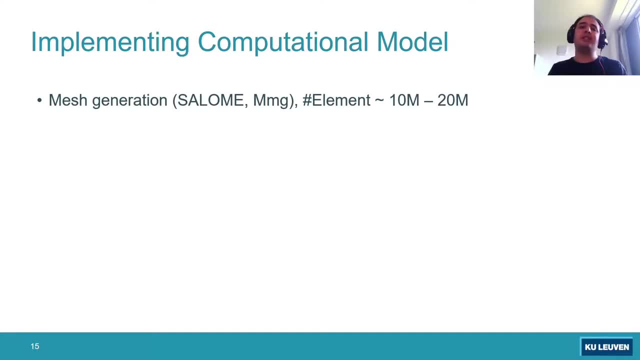 we usually end up with 10 to 20 millions of elements, So quite a large number of elements And for degrees of freedom. so when we want to implement it in software, in programs like FreeFEM, for weak formulation, and then you know to assemble the linear system of equations to solve for each. 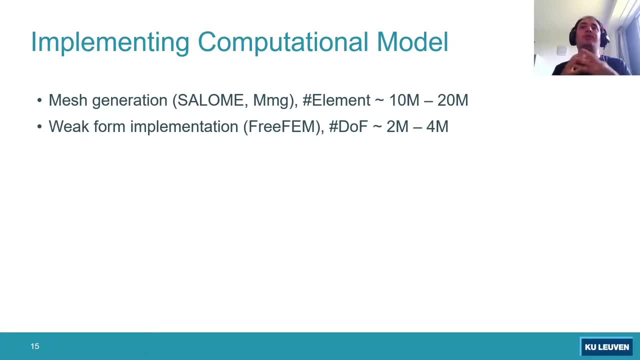 PDE, we have a degree of freedom of 2 to 4 million. So that's actually how it works in practice And this is the reason that parallelization is essential actually for this work. So we employ a, you know, combination of two techniques: high-performance domain decomposition and also high-performance. 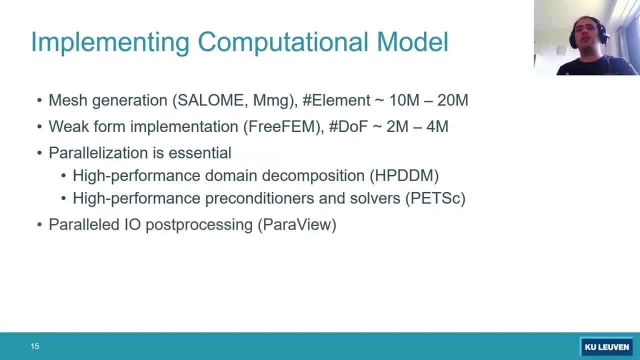 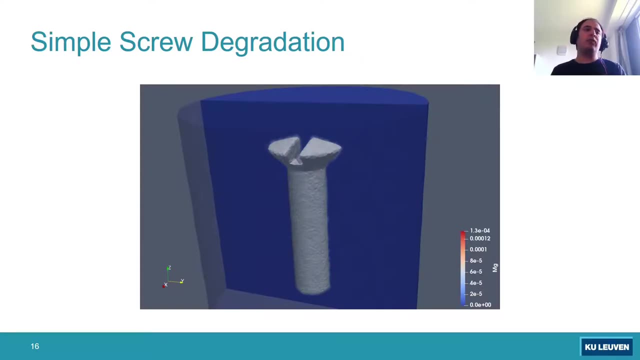 preconditioners and solvers and also the IOD. the input-output of the results is in a parallelized way for parallelized post-processing. So these are some, you know, a quick overview on some of the results that we have on this. 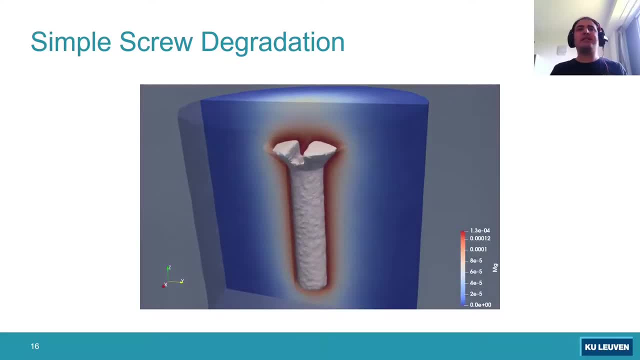 So this is a simple screw degradation. You can see that together, that the white interface evolving is actually shrinking is the corrosion front which is captured by level set, and you can see the release of materials to the surrounding and also the way that. 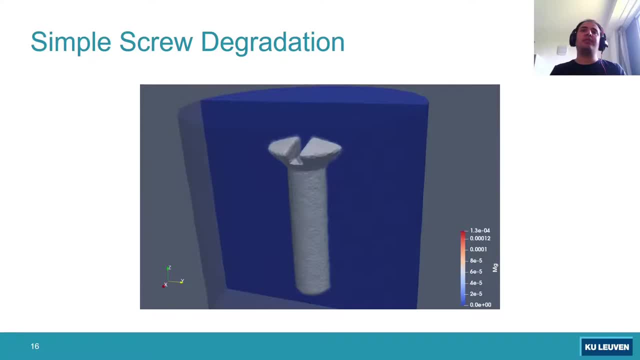 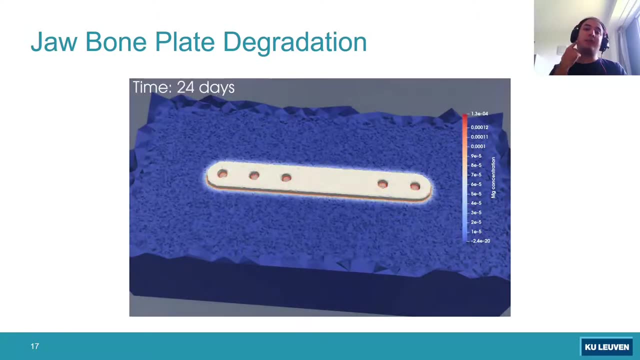 we can capture the topology changes, the shape changes during the degradation simulation. This is a simulation for a jawbone plate- degradable jawbone plate that is degrading. You can see the release of material and also shrinking of the surface. 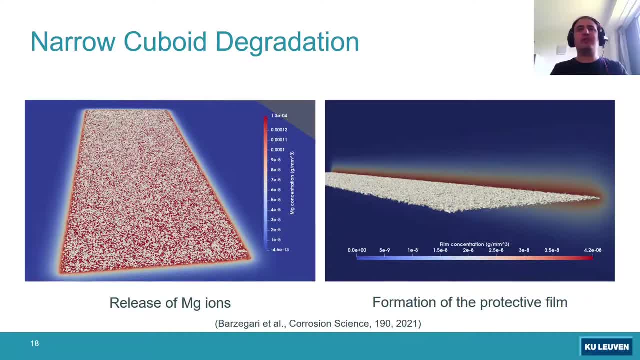 And this is of you know to. this is for mostly for validation of the models, the release of magnesium ions and for the animation of a protective film on a surface. As I said, this is something that is captured by the model and this is another. 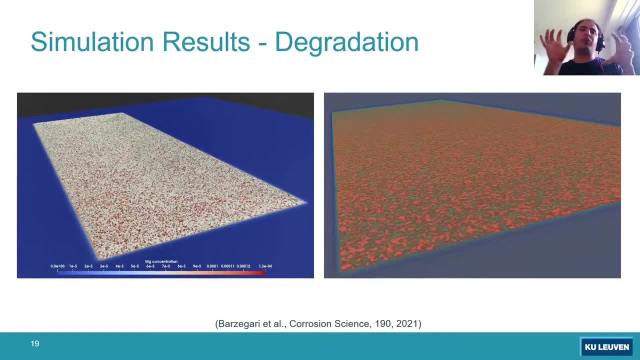 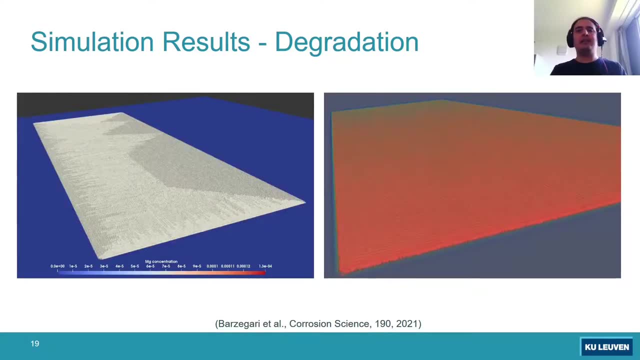 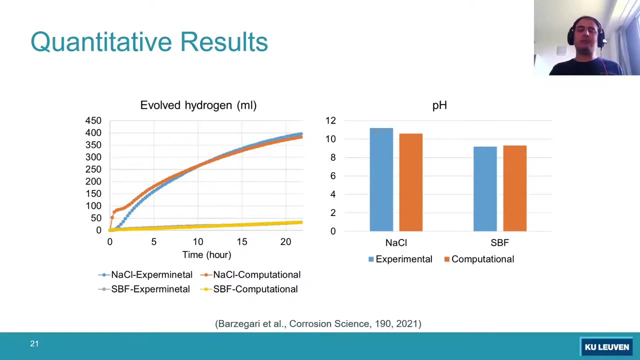 animation of degradation that are post-processed in two different ways. You can see the release of material and the way that the metallic block disappears. And from the quantitative perspective, we have compared the side corrosion, product formations, in this case evolved hydrogen, as well as change of pH, with the experiments, with the dedicated experiments that were performed. 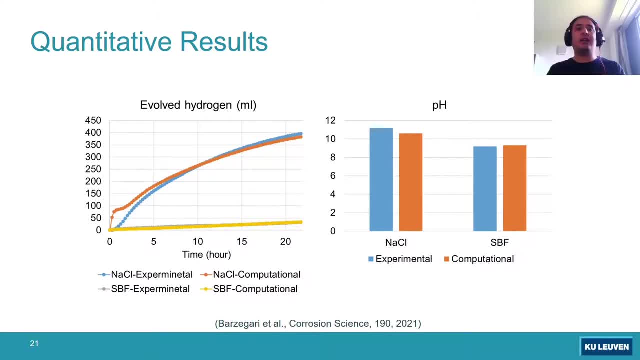 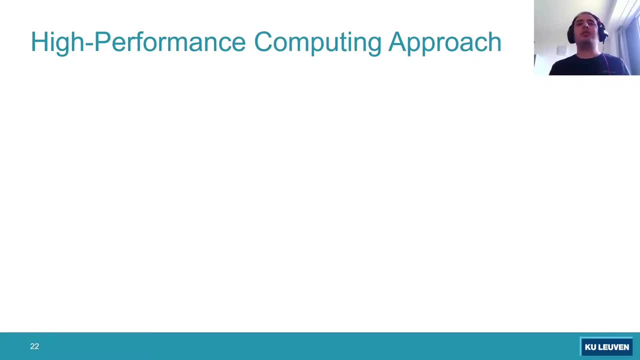 with the computational models And you can see that they are in a good agreement, actually, Okay, as I said, this has been achieved using HPC, because otherwise the simulation could have taken ages to complete, and I want to show you some more details on the parallelization approach that we employed. It includes first the 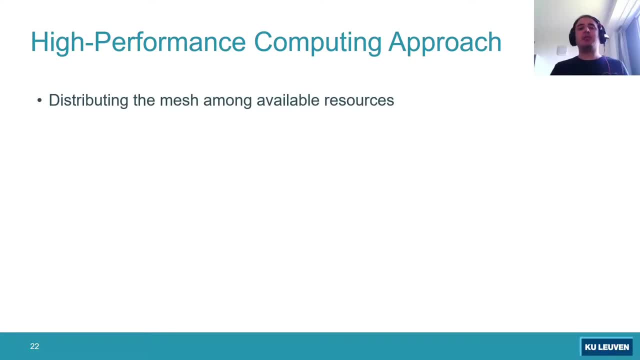 distribution of mesh among available resources or sort of mesh decomposition, which has been done using overlapping Schwarz method, and also solving the linear system of equations. A finite element, you know, leads to a linear system of equations. In this case it consists of, you know, millions of unknowns and we use algebraic multi-grid. 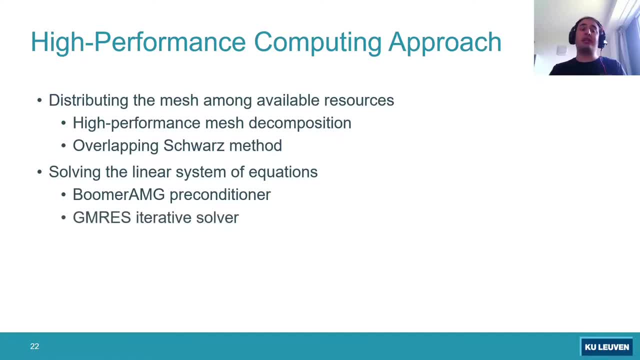 preconditioners for reaction diffusion systems, and then GM res iterative solvers to solve the system, as well as field-displeted preconditioner for Floyd-Fuller and Navier-Stokes equations. So the way that the mesh decomposition works is actually, as I said, using overlapping Schwarz. 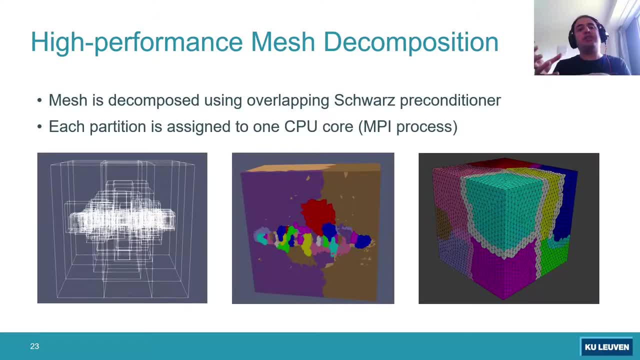 preconditioner. and then you know it's a sort of mesh partitioning, and then each partition is assigned to one CPU core for parallel processing. And these figures belong to a simulation with 170 CPU cores, or let's say MPI nodes. 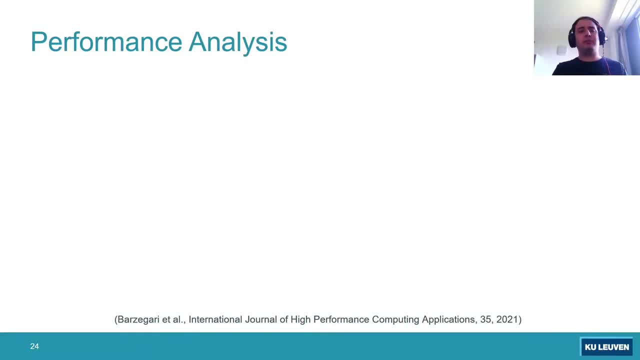 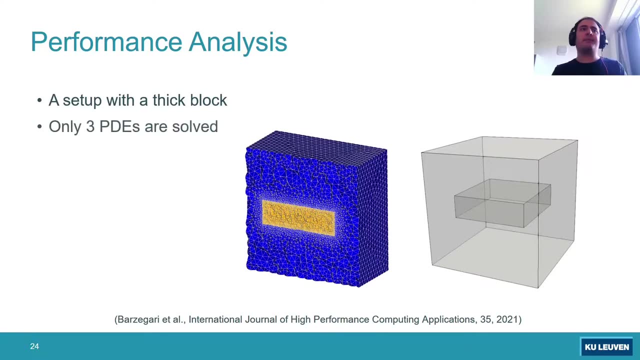 So for performance analysis we did a, we did a sort of benchmarking on a simpler and a smaller system, So a setup with a ticker box in which we solved only three PDs out of eight or seven, as I said, And then degrees of freedom for each PD is around 150,000, and then the number of elements around 1,900,000. 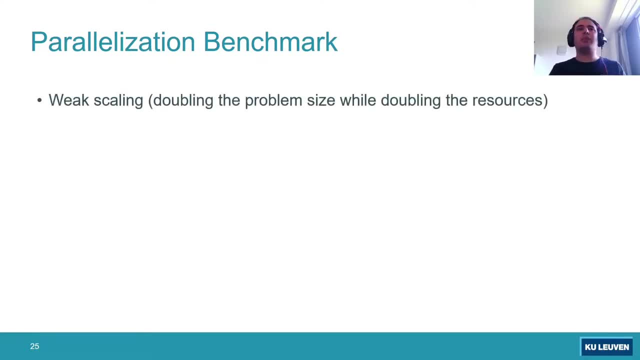 And for benchmarking we used wicket scaling, in which you double the problem size by doubling the resources, so the execution time ideally should be the same. So this is a demonstration of that. You can see that we double the problem size. 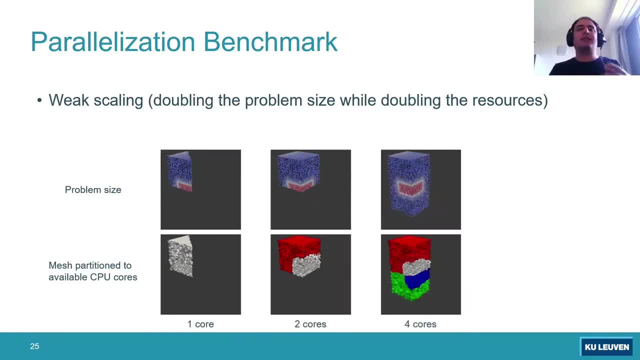 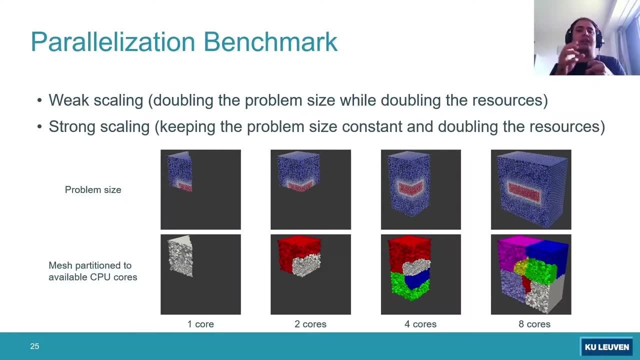 while doubling the cores as well. So you know, this is how wicket scaling works, And also strength scaling, in which you keep the problem size constant and you double the resources in each. you know, in each, in each stage, And ideally the performance should be doubled. 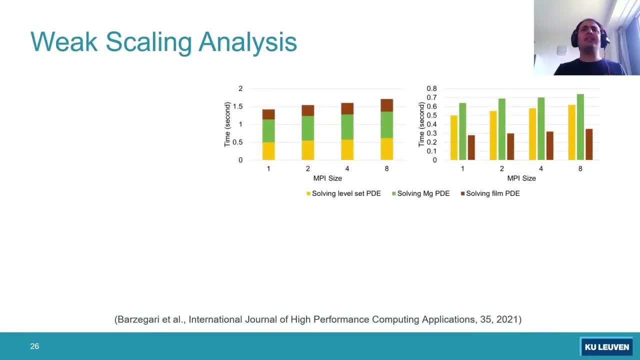 in this test. So for wicket scaling results, you can see that the performance would be up to eight cores to see how it works, And this is the speed-up and parallel efficiency, a proper parallel efficiency, And to analyze this, actually, the common rule is actually: 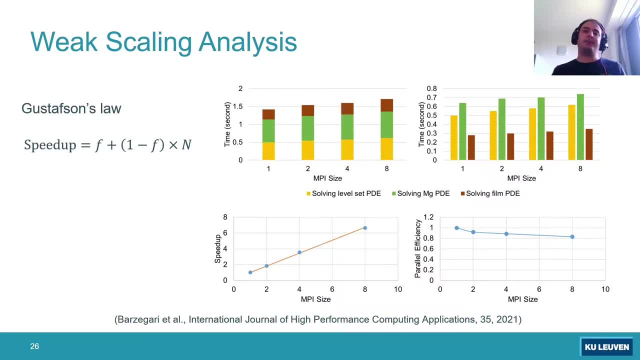 Gustafsson rule in which you have, you know, an ideal performance, an ideal speed-up, And then, by interpolating this line on the speed-up results that you have, you can compute the sequential part and parallel part of the code. In this case it was 82%. 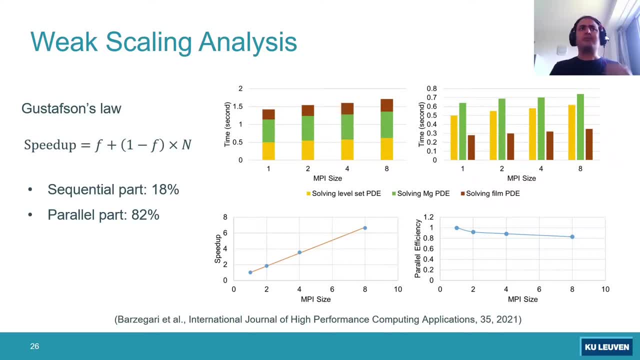 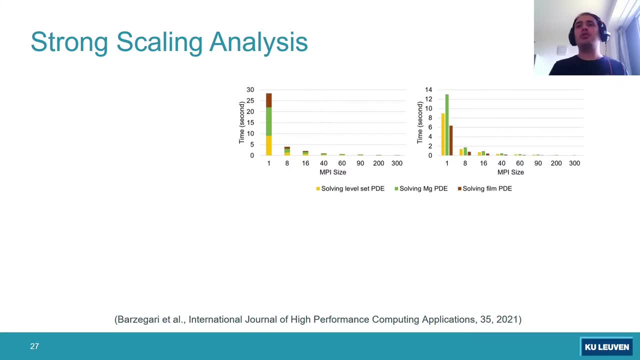 of parallel part And also for strength scaling. you can see that we have performed the simulations to up to 300 cores. And then for speed-up and efficiency. you can see that efficiency is almost half with 300s, which makes sense because you have overhead in lots of things for memory overhead, for communication overhead and this kind of stuff. 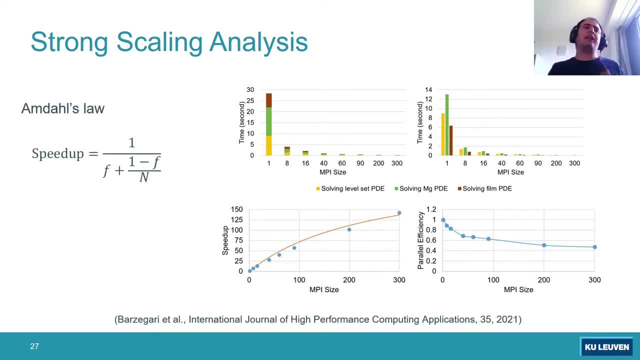 And the common rules that is usually used is Amdahl's rule with a different equation, So with an interpolating equation, we will have the sequential part, which is actually the value of f here, and the parallel portion to be 99% and 1%. So it shows that the code has a high potential to be parallelized. 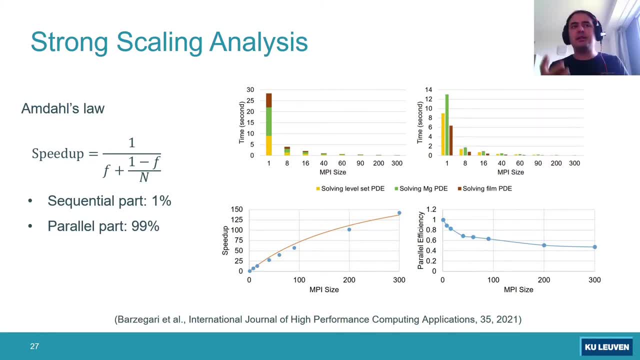 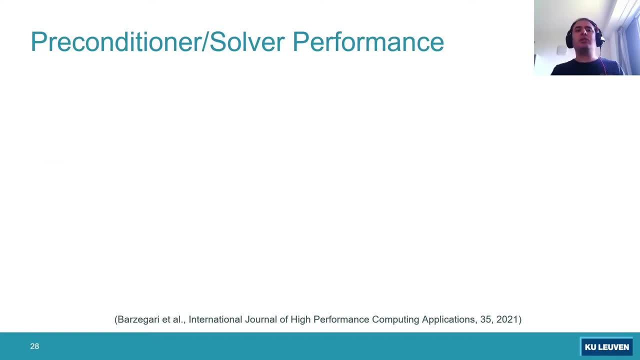 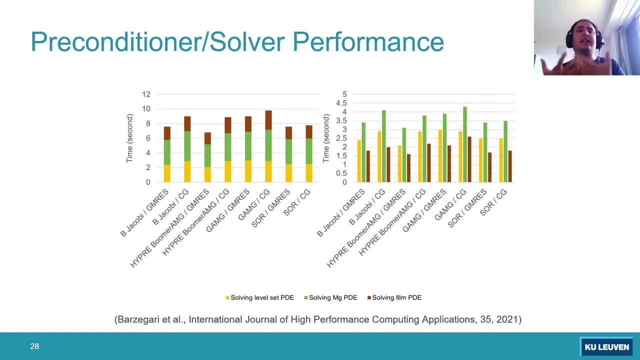 And besides the speed-up and efficiency, we can see that the employed technique is actually a good scaling performance And also for preconditioner and solver performance. as I said, yeah, we have compared different preconditioner and solvers and in the end we came up with 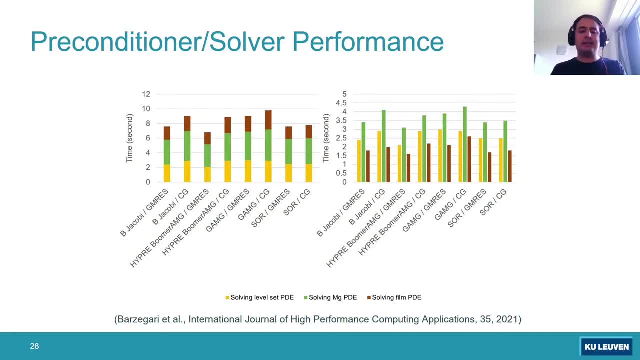 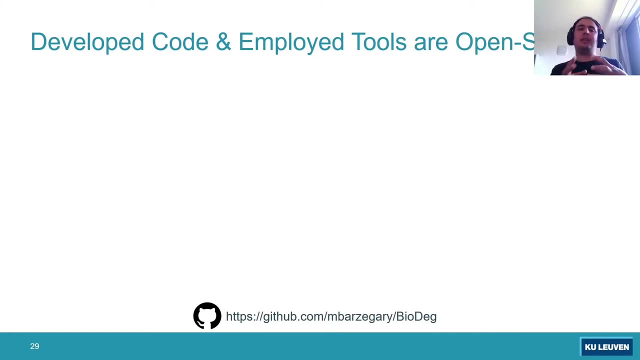 the algebraic multigrid and GMR solver, and that's actually the reason that we saw the best performance is this shift, using this combination. And, as a final note, I can say that all the developed codes and employed tools are all open source, so I have used a wide range of different libraries and tools. 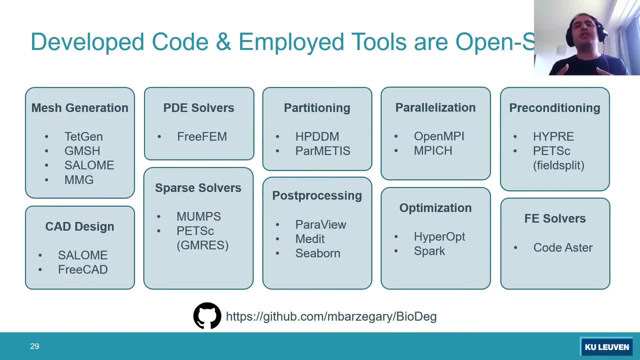 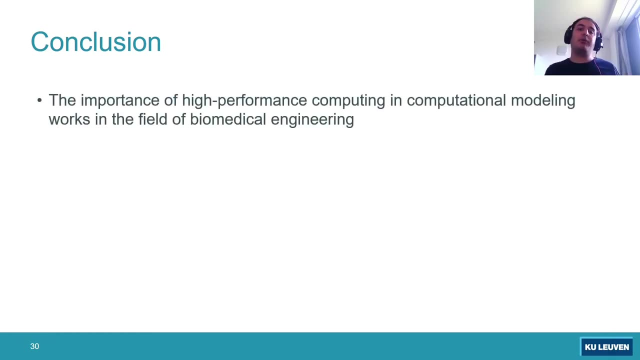 for in this research, but they are all open source And, as a result, the final code that we have developed is also open source and freely available on github, so you can check it out if you are interested. So in this presentation we talked about the necessity and portents of high performance computing.